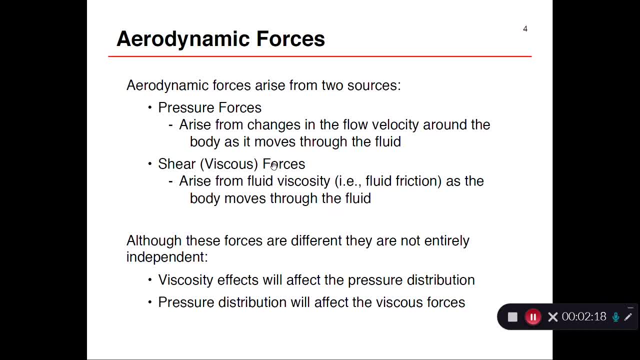 down. So we have two type of forces that we need to worry about. They are not independent. If the viscosity causes the boundary layer to grow, which changes the effective shape of the body, perhaps even cause the body to stall, changes the pressure distribution. Likewise the pressure. 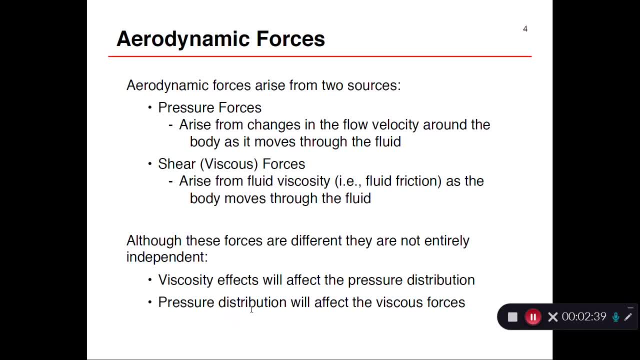 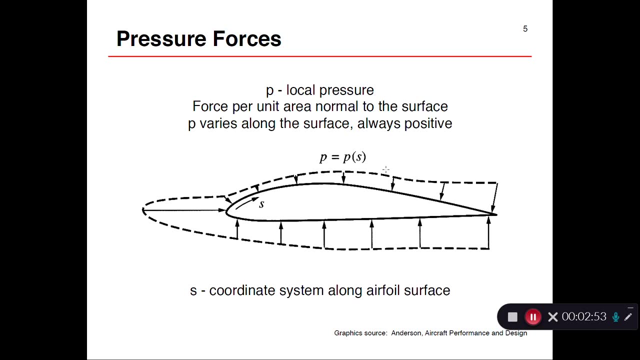 distribution. if you have an adverse pressure gradient, that means the pressure is rising. the boundary layer may get separated. So these are not really two different phenomena. They are interconnected to each other. So one way of visualizing the pressure is to plot arrows. If it is pointing towards the body, it's a positive pressure, the positive gauge pressure. 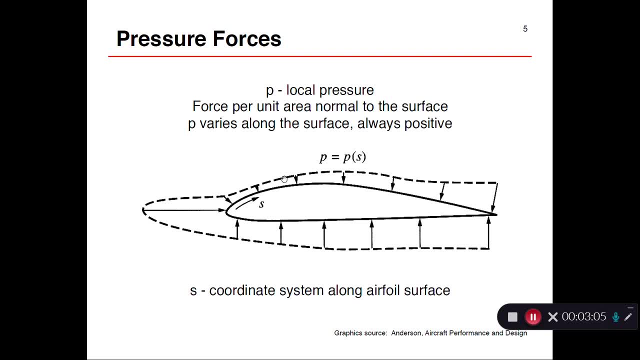 If it is away from the body, that means negative gauge pressure. What do we mean by gauge pressure? Gauge pressure is P minus P atmosphere. That's what a pressure gauge will measure. So if you have a regular, if you have a, if you don't have a P, infinity subtracted from it, P is always going to be positive. 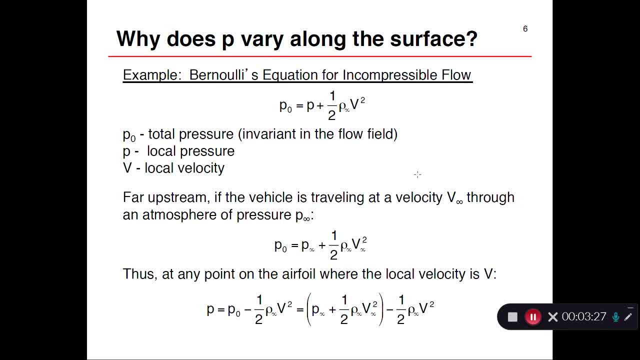 It's going to be always pointing towards the body. So why does P vary along the surface in an incompressible flow? Bernoulli equation says: when the pressure energy goes up, the kinetic energy goes down, and vice versa. So pressure and velocity are changing. 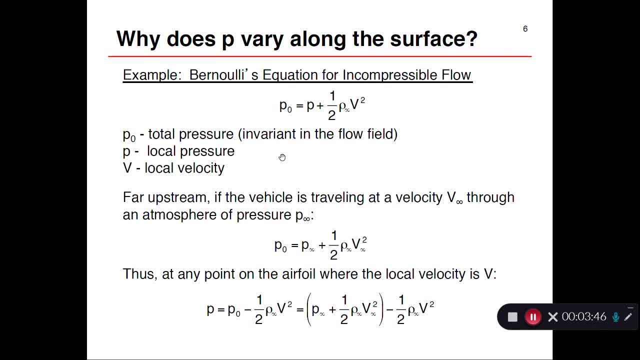 When the velocity changes, pressure changes. When the velocity changes, pressure changes and vice versa. Incompressible flow. you have something more complicated. Cp times T naught equal to Cp times T plus one half: rho V squared. Cp times T plus one half: just V squared over V squared. 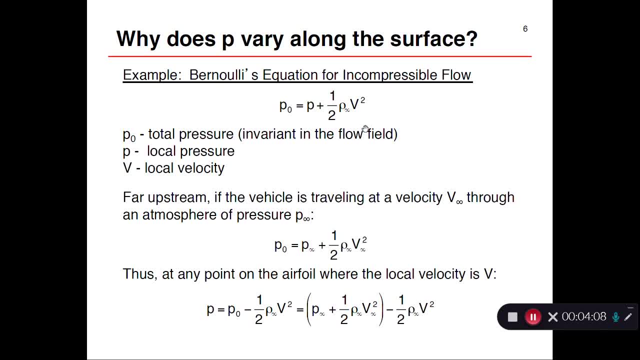 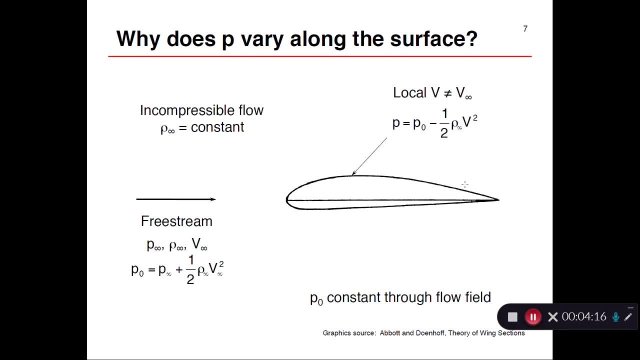 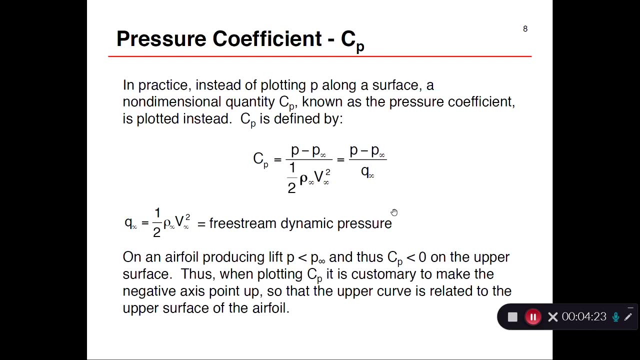 There's no rho. Then when the temperature goes up, velocity goes down and vice versa. So why does the pressure vary along the surface? Because the body disturbs the flow. So all over the body the velocity is changing. Now non-dimensionalization of the pressure is, as we mentioned, gauge pressure, which is P above the atmospheric pressure divided by the dynamic pressure. 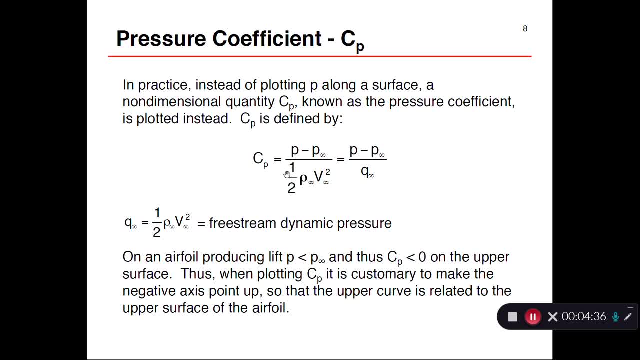 This is sometimes called Q. Therefore this would be called a dynamic head. So this is Q. So on an airfoil, some places P will be greater than P. In 3D Cp is positive, Other places it's negative. 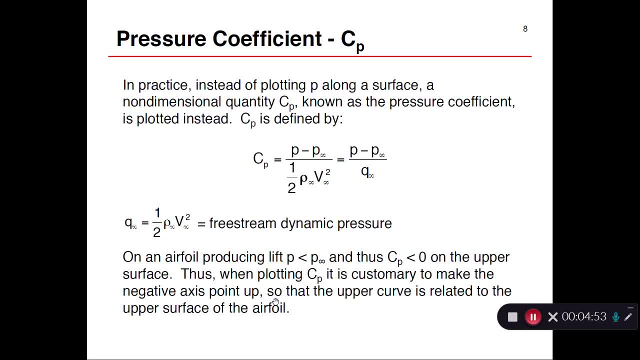 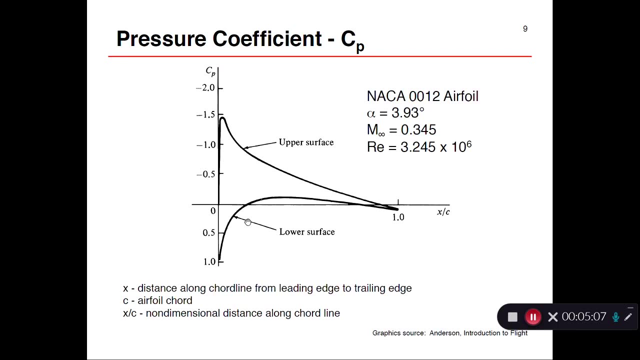 Since Cp is non-dimensional, we will also non-dimensionalize the distances. For example, for an airfoil we will measure the distance along the chord line and divide it by the chord so that it goes from zero to one. So this is a picture of X over C, nose of the airfoil to the trailing edge of the airfoil. 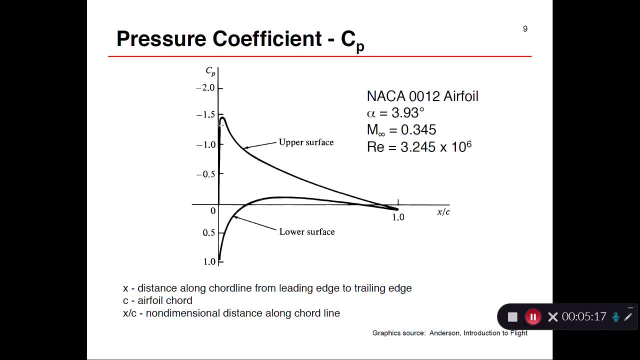 Cp goes from positive to negative, So very high. positive value means P is very, very high compared to P infinity. Negative value means P is less than P infinity. So over a very, very short distance from the nose of the airfoil, from the front stagnation point, pressure rapidly decreases. 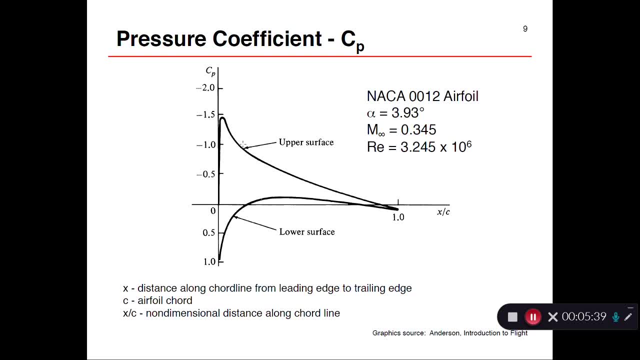 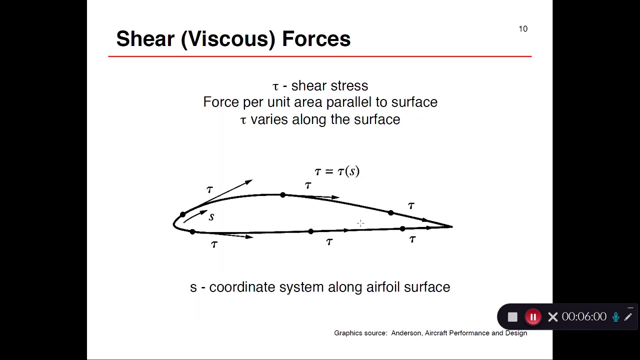 Then it starts increasing. So this is what we call an adverse pressure gradient region. On the lower surface. something more or less similar happens, but not quite so dramatic: rise, not quite so dramatic pause, fall. Now the difference in the pressure between the upper and lower surface. essentially, this area is a measure of the lift coefficient. 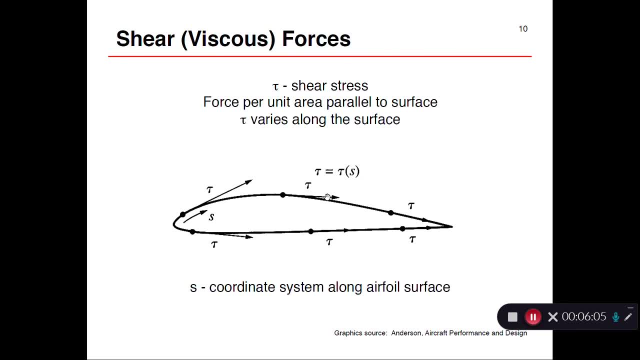 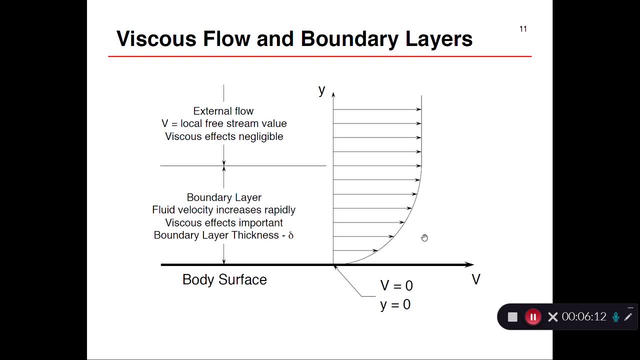 How about the viscous drag? Shear stresses are tangent to the surface. Therefore, we should be integrating along the surface. So we would, If you know, have some knowledge of the boundary layer from our aerodynamics class. this is the slope at the body surface, is the velocity gradient. 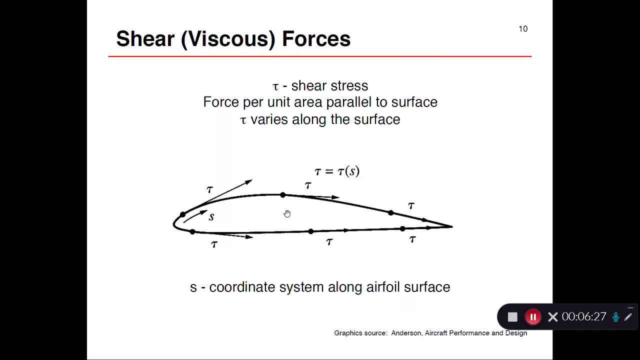 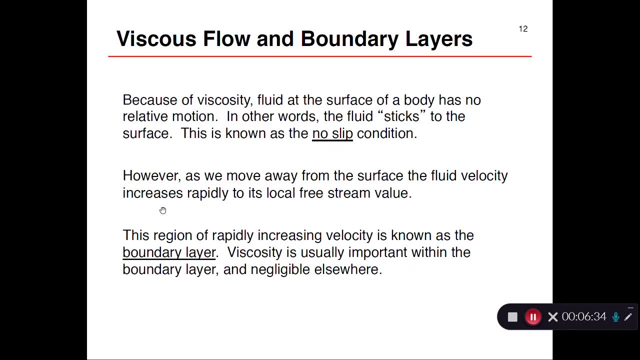 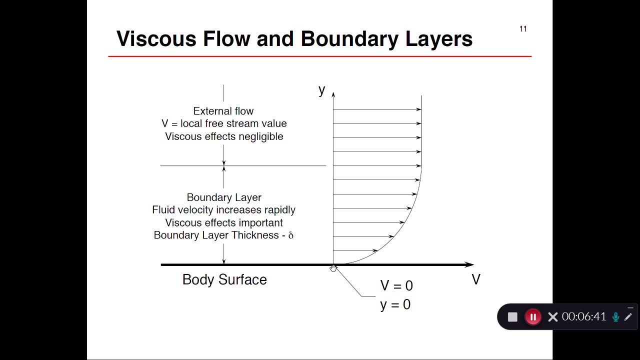 If you multiply by molecular viscosity, that gives you this tau. So once you have the molecular tau, you could integrate it all over the body surface. Because of viscosity right at the body, the molecule come to a complete rest. At the edge of the boundary layer molecules are moving at the local potential flow velocity. 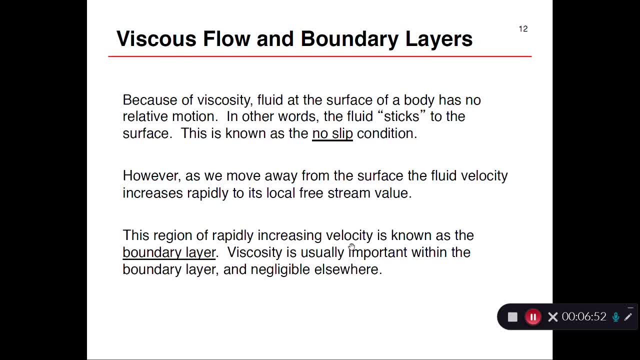 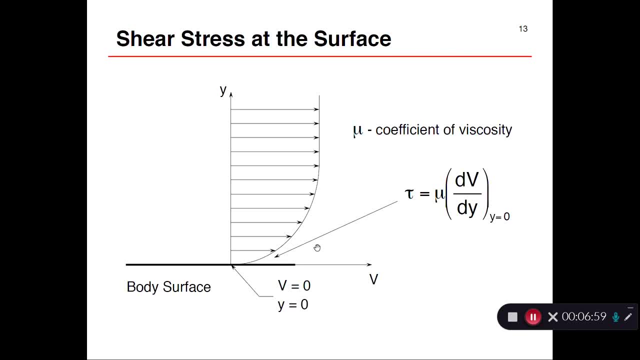 So velocity is changing like this. This: we saw all these concepts in the aerodynamics course. Now the slope at the wall multiplied by viscosity is called the shear stress. This is the Newton's. When Newton first found the shear stress, he found: 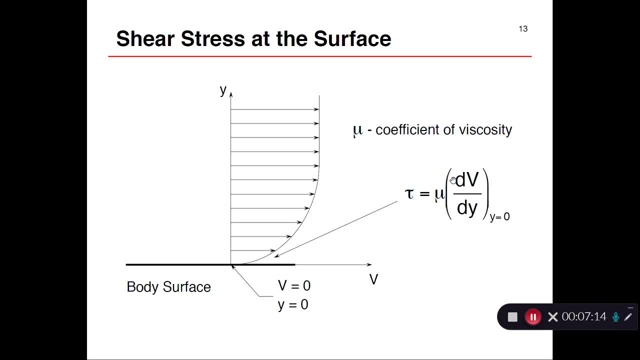 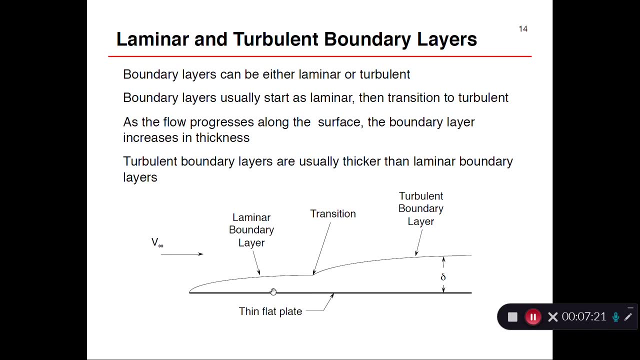 Viscosity times the velocity gradient: Velocity over distance. Now, if you have a laminar flow, you are going to have a lower shear stress at the wall, lower drag in general. When you go to turbulent flow, you are going to have a higher shear stress, higher drag. 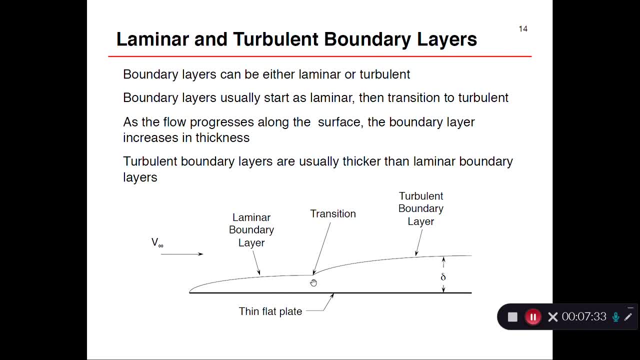 So the region where the flow goes from laminar to turbulent is called a transition regime. There the boundary layer abruptly starts growing very, very fast. All these concepts we would have seen in the aerodynamics course. We are just recapping it here. 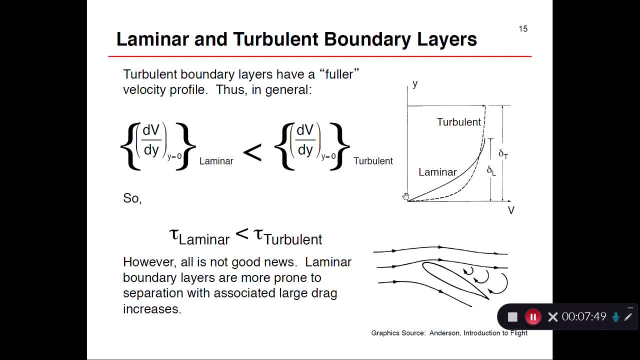 So the laminar slope, this slope, Think of it as this is the horizontal line, This is a curve Slope- is this angle included angle between the y-axis and the velocity profile. So if this angle increases, that means the slope is higher. 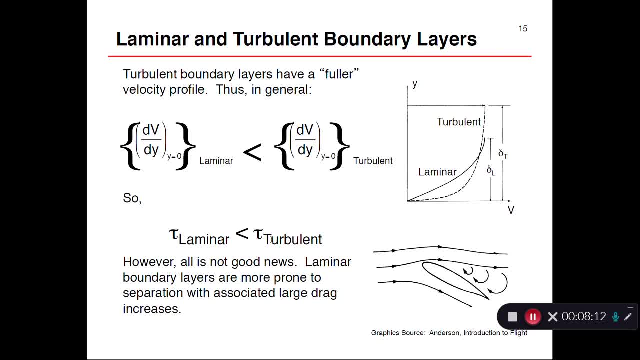 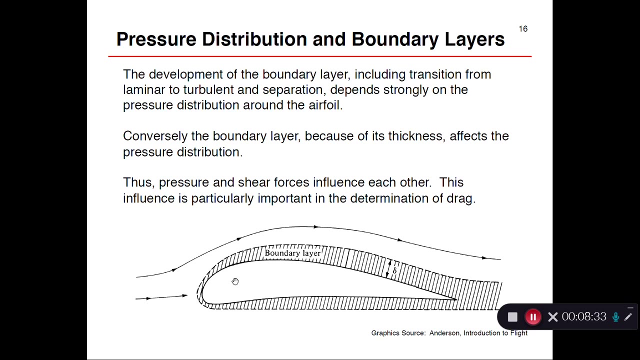 So turbulent flow has got a higher slope. Higher drag is bad from a drag perspective But stall may be reduced because of the extra mixing of the turbulent flow. So you may get improved stall characteristics in turbulent flow. So you have a pressure distribution and you have a shear stress distribution all over the surface. 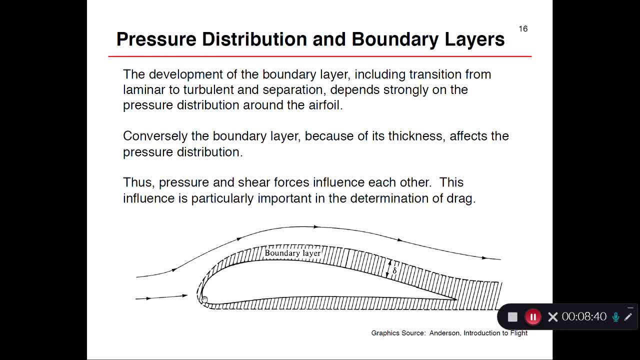 This is the boundary layer thickness. Boundary layer changes the effective shape of the body. Therefore it changes the potential flow. Potential flow or the pressure distribution changes the velocity profile, Boundary layer thickness. So these two are interconnected. Coming back to our shear stress, it is tangent to the surface. 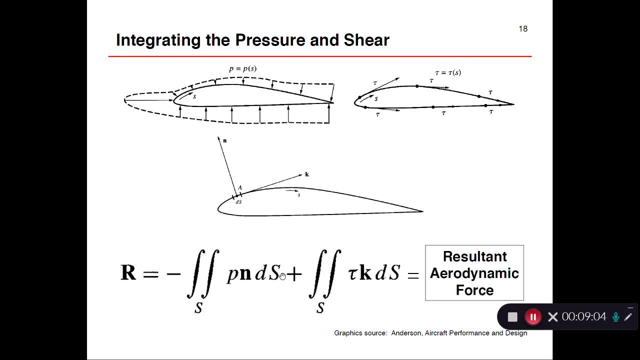 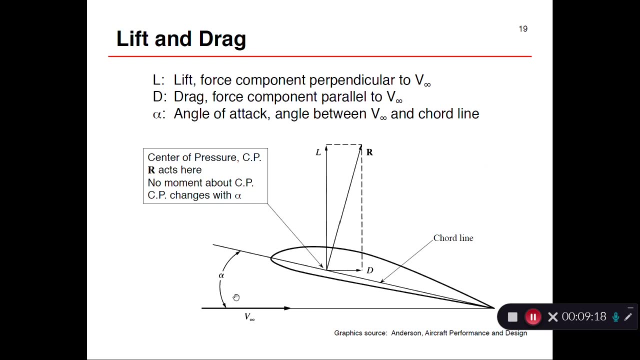 Pressure is normal to the surface. So when you integrate it you multiply the pressure by the normal vector, your shear stress by the tangential vector, Then you will get a vector force. Lift is normal to the V infinity. Drag is along the V infinity by convention. 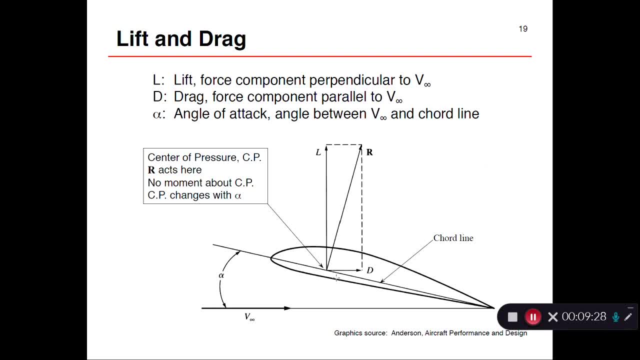 Center of pressure is the point where you have a no moment. It is not a center of gravity which deals with masses. This is the you may think of it as a center of pressure. At this point, there is no moment. Aerodynamic forces pass through this point. 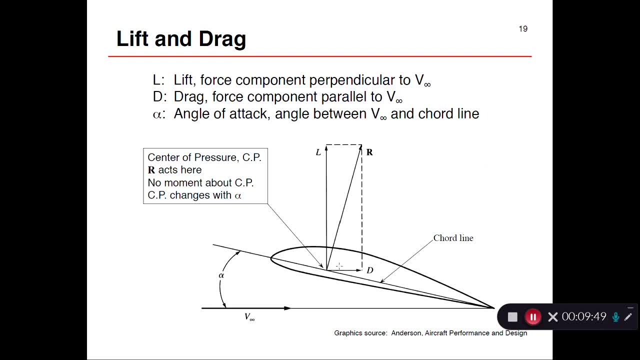 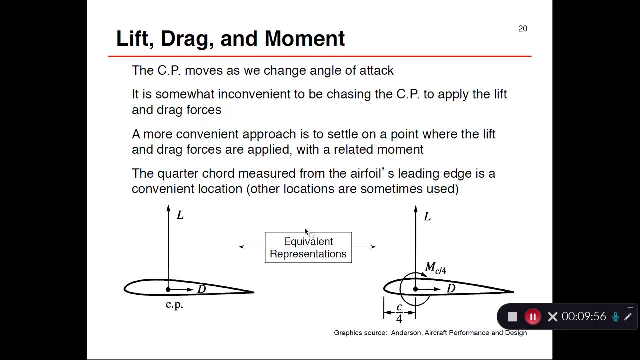 But there is no moment at this point. Unfortunately, the center of pressure changes with the angle of attack alpha. Therefore we define, sometimes called an aerodynamic center, usually at the quarter chord. At the quarter chord the pitching moment, no sub-pitching moment. 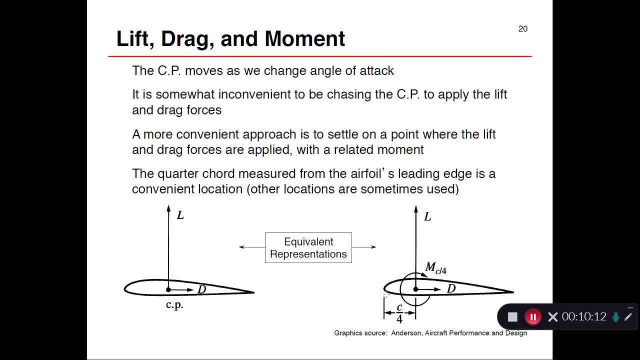 is caused by the aerodynamic forces is independent of alpha. So the point on the body where the pitching moment is independent of alpha is called the aerodynamic center. So that aerodynamic center usually occurs at the quarter chord. These concepts we see in aerodynamics course. 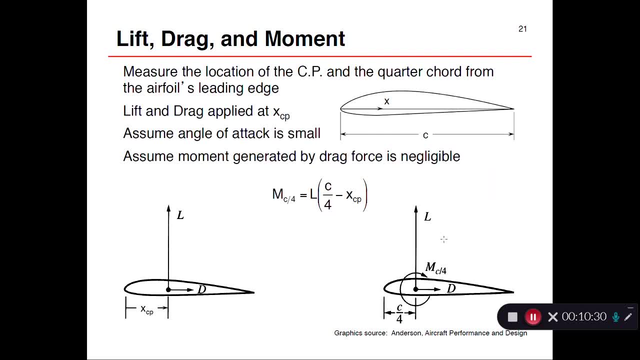 And we see it here again. Now, if somebody gives you moment at the quarter chord, at the center of pressure, this moment is zero. So moment at the quarter chord point would be simply the distance between the center of pressure and the quarter chord point. times lift. 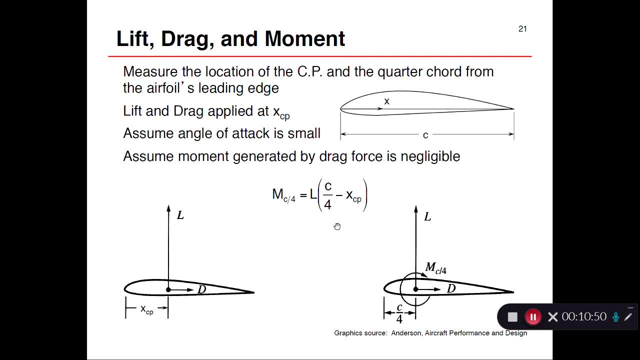 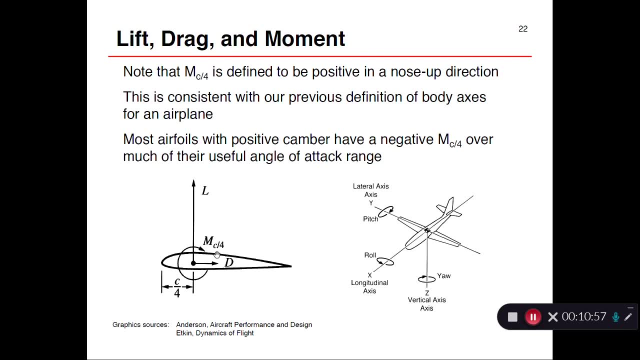 That will be the moment. So moment is here. we are talking about simply in the two-dimensional direction, But in the aircraft geometry you would have a rolling moment, pitching moment, yawing moment of a complete aircraft, as we saw earlier. 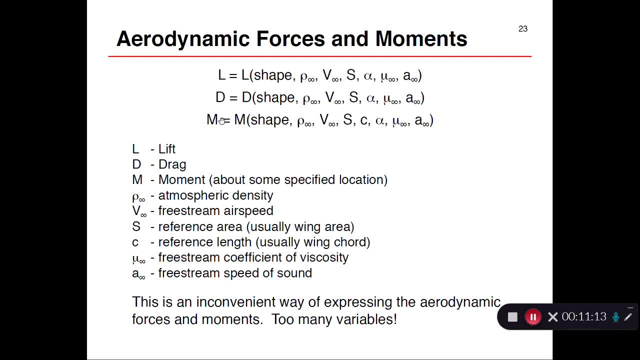 Now for a complete aircraft lift, drag and pitching moment would be a function of the shape of the geometry: density, velocity, wing area, angle of attack, viscosity, speed of sound. So this is a dimensional grouping, So we want to scale it. 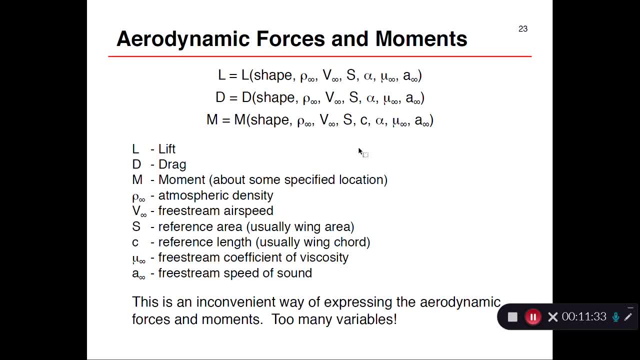 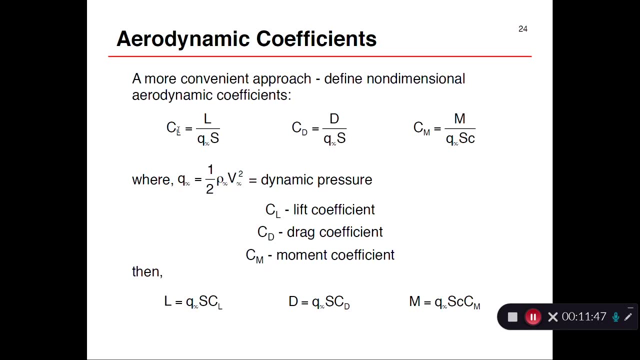 So we could test a scaled model or maybe do an analysis of a CFD analysis or an aerodynamic analysis of a scaled model. So we want to non-dimensionalize all these dimensional quantities. So what do we do? We non-dimensionalize lift force. 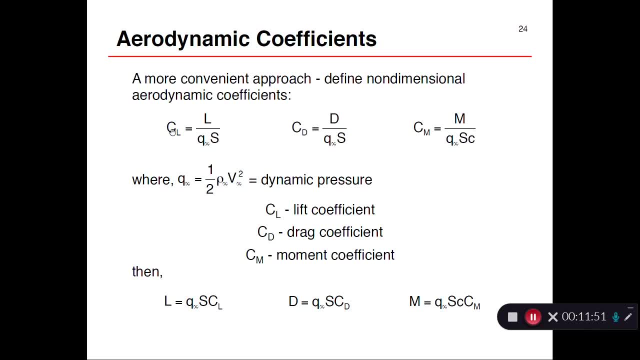 divided by Q infinity times wing area. We call it CL. Drag is Q infinity. Yes, our numerator is drag. Moments usually have an area times distance, So you have to put a distance which is a reference distance If it's a 2D aerofoil. 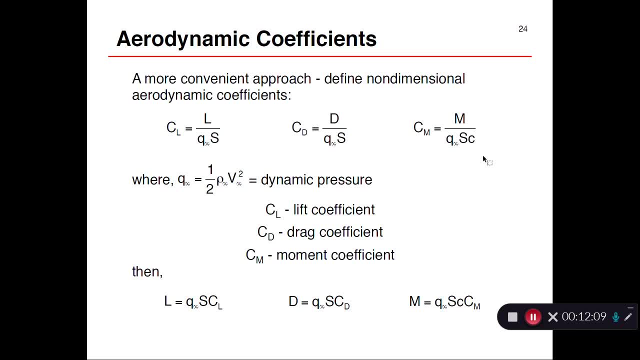 it's a local chord. If it's a 3D airplane, you have to agree on what this reference length is. Is it a wingspan? Is it a root chord? Is it a tip chord? You have to come up with a commonly agreed to definition. 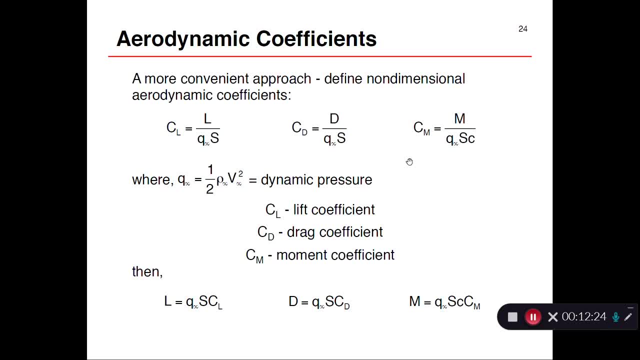 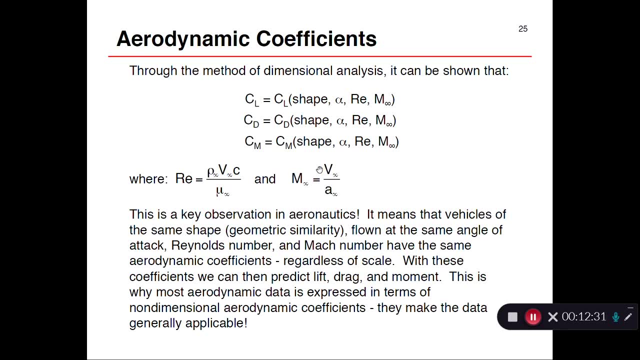 Then you base your CM based on the particular definition. This is the Reynolds number, This is the Mach number. We have seen this before, So we could now write, instead of a dimensional number, non-dimensional quantities. scaled body, not an actual body. 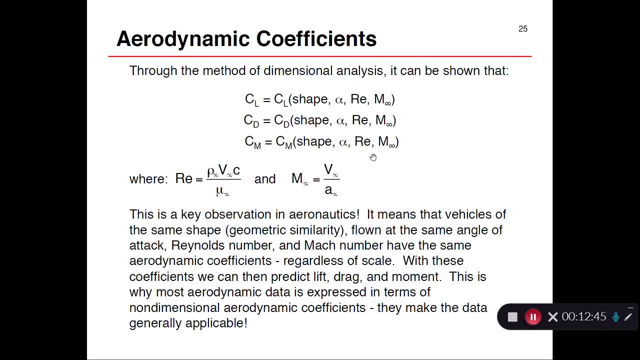 non-dimensional alpha, non-dimensional Reynolds number, non-dimensional Mach number. Wright brothers realized the power of scaling, So they tested everything in a wind tunnel. They built a small scale model and computed CL, CD and CM. The rest of the world was using this equation. 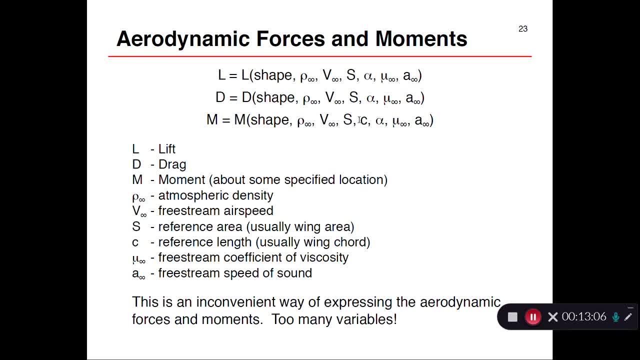 That means they were building a full scale model, for example a full scale glider, and they will jump off a cliff and see what happens. Some live to tell the story, Others are written in their obituary in the Atlanta Journal of Constitution. 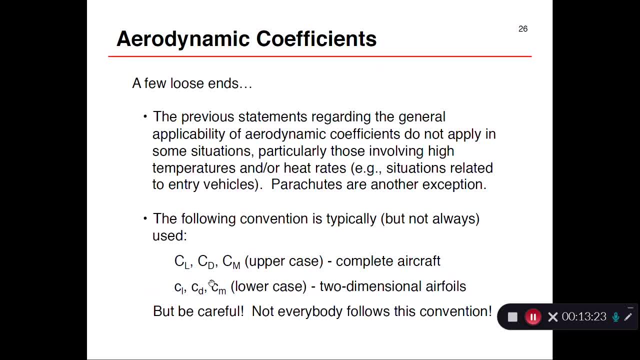 So a few loose ends: Lowercase ldm is for aerofoil, Uppercase ldm is usually for aerofoil, Uppercase ldm is usually for airplanes. So this is a convention. We will use some books, some notes.